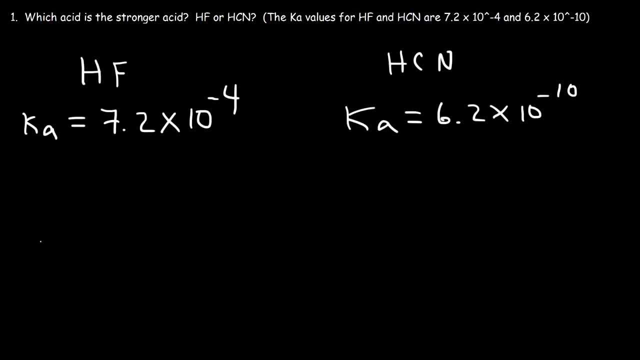 acid. Now you need to know that acid strength increases with increase in Ka values. So the acid with the higher Ka values is 7.2 times 10 to the minus 4.. So you need to know that acid strength increases with increase in Ka values. So you need to know that the acid with the higher Ka values 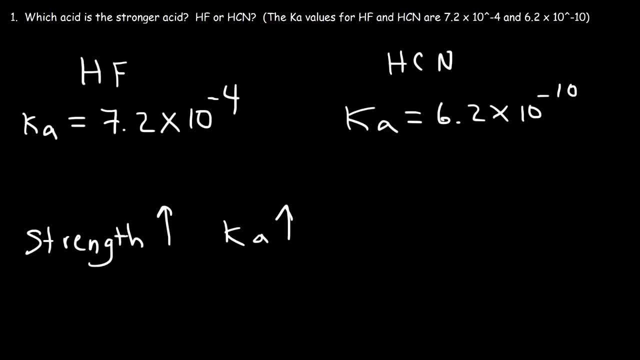 is going to be the stronger acid, And since 10 to the minus 4 is greater than 10 to the negative 10, HF is therefore a stronger acid than HTN. So this is the answer. Now, what about number two? Which oxy acid is stronger, HNO2 or HNO3?? The answer is HNO3.. HNO3 is HNO3 or HNO2.. HNO2 is quite different. HNO2 is HNO3.. HNO3 contains HNO2. вечerine HNO3 also contains HNO2, a clear form of concentration. When you Г, does HMO3 contain alpha-opendehyde? 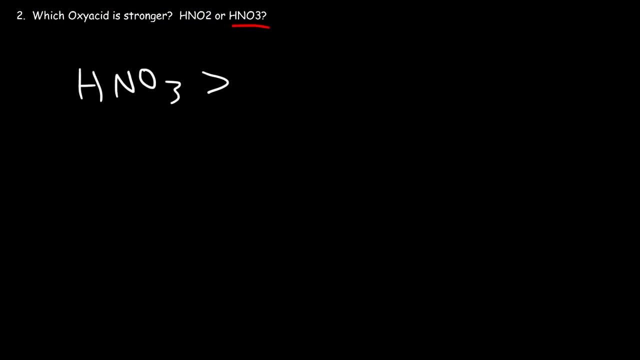 HNO3 is stronger than HNO2,. it has a higher Ka value Now, so you need to know this. for oxy acids, the acid with the greater number of oxygens is typically the stronger acid. So, for example, HClO4 is a stronger acid than HClO3, and this is stronger than HClO2, and 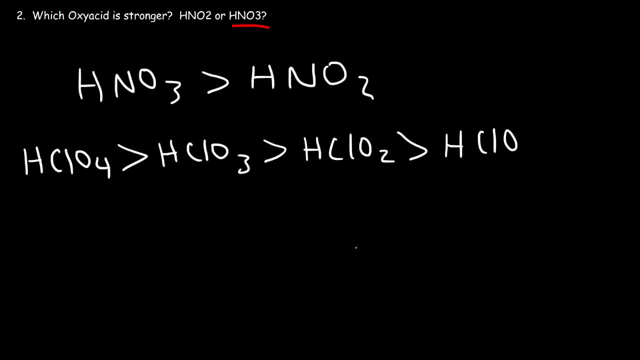 this is stronger than HClO. Now, HCl doesn't fit this trend. in fact, HCl is stronger than Ni3. So you can't put HCl in this trend. it doesn't have an oxygen, it's not considered to be. 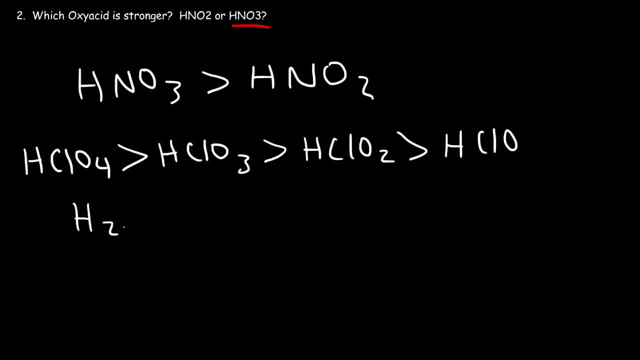 an oxy acid, But for other oxy acids, like H2SO4,, this is a stronger acid than H2SO3. So the trend works for oxy acids, only those that contain oxygen in it. Now let's move on to our next problem. 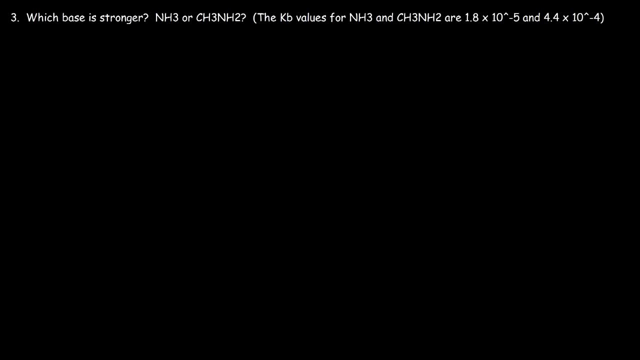 Number 3, which base is stronger? Is it ammonia or methyl amine? Ammonia is NH3, methyl amine is CH3NH2.. Now we're given the Kb values of these two bases. this is the base dissociation constant. 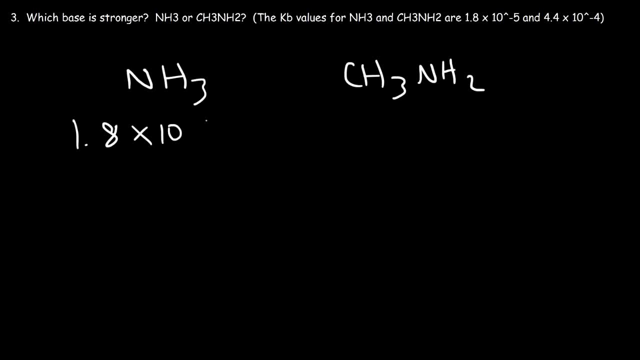 And so the Kb for ammonia is 1.8 times 10 to the minus 5, and the Kb for methyl amine is 4.4 times 10 to the minus 5.. So the Kb for ammonia is 1.8 times 10 to the minus 5, and the Kb for methyl amine is 4.4 times 10 to the minus 5.. 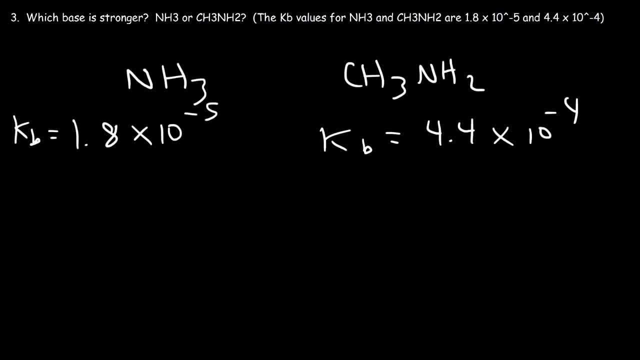 So, given this information, which base is stronger? Now, you need to know that base strength increases with higher Kb values. these two are proportional. So which value is higher- 10 to the negative 5 or 10 to the minus 4?? 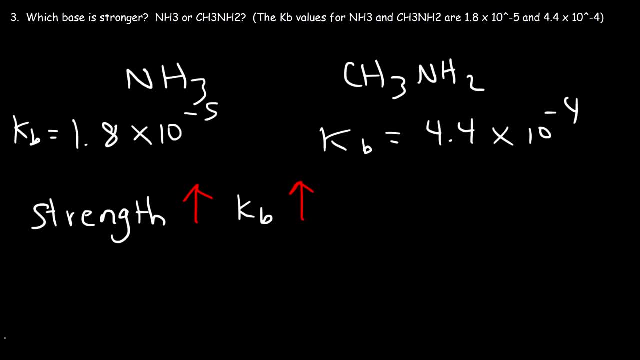 Negative 4 is higher than negative 5 on the number line. So let's say, if you were to draw a number line, here's 0. This is 5, here's negative 5. The higher numbers are on the right side. so negative 4 is higher than negative 5, which. 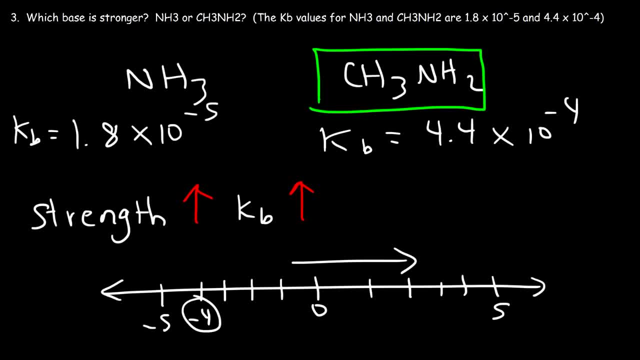 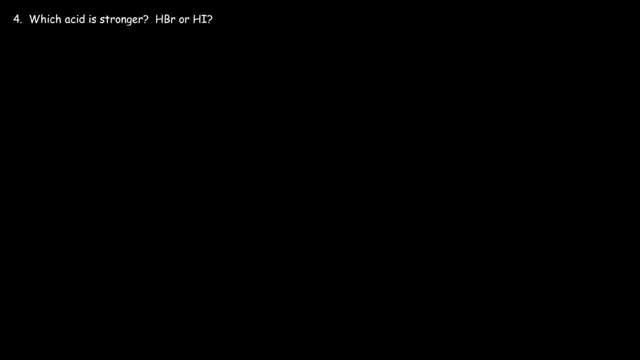 means that methyl amine is the stronger base because it has a higher Kb value. Now what about the next one? Which acid is stronger? Is it HBr or Hi Hydrobromic acid or hydroiodic acid? And how can we find the answer without knowing any? 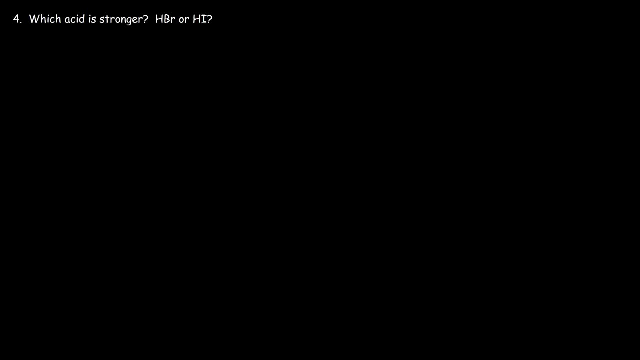 Now you need to know the trend for acids. So let's say this is carbon, nitrogen, oxygen, fluorine, chlorine, bromine and iodine. So these are the elements in the periodic table. Acid strength increases as you go to the right and as you go down. 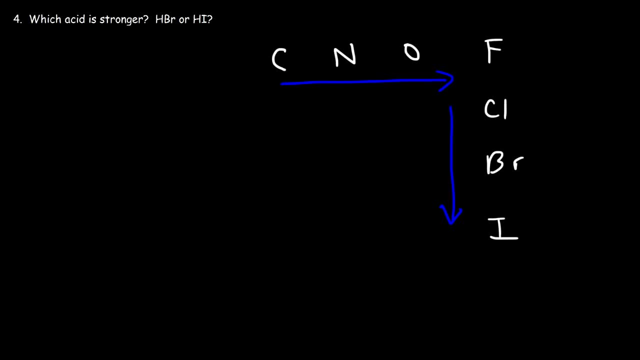 For acids if hydrogen is directly attached to these elements. if it's not, then this trend may not apply, So keep that in mind. So this is for binary acids. So what this means is that HI is a stronger acid than HBr, which is stronger than HDL. 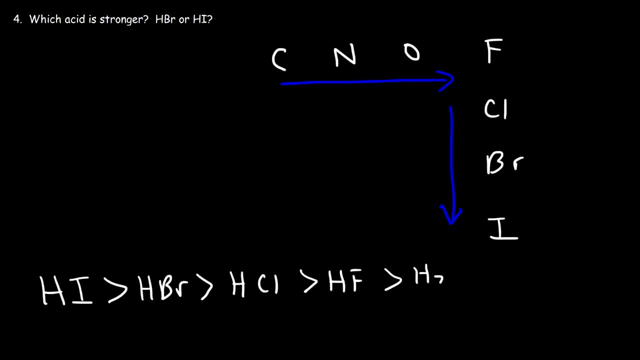 and that's stronger than HF, and HF is stronger than water. water is more acidic than ammonia and ammonia is more acidic than methane. So that's the trend for the binary acids when H is directly attached to the element itself. So, comparing HBr and HI, you can see that HI is stronger than HBr. 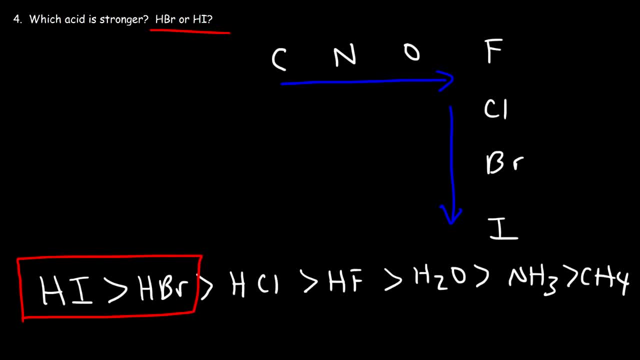 So what does this mean? It means that HBr is stronger than HCl. HCl is stronger than HCl. HCl is stronger in acidity than HBr. So HI is the answer, that's the stronger acid Number five. which acid is stronger, HOCl or HOI? 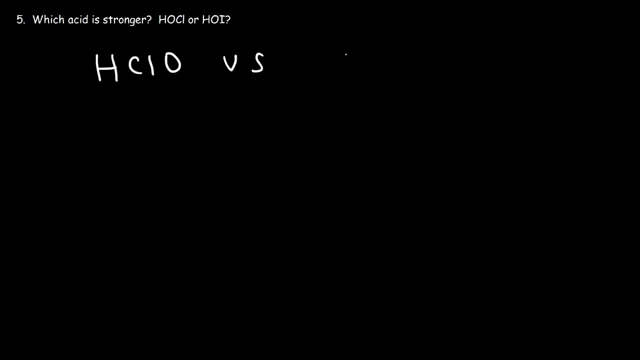 You can also write it as HClO- hypochlorous acid- versus HIO- hypoiodous acid. So which one is stronger? Now recall the trend for the binary acids, where we said that HCl is stronger than HBr. 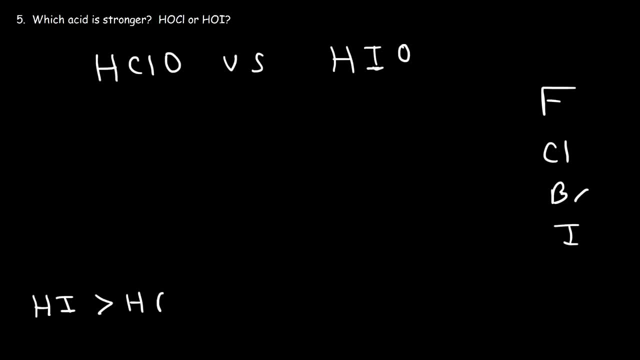 HI is a stronger acid than HBr, which is stronger than HDL, which is stronger than HF. So HI is more acidic than HDL, That's if hydrogen is directly attached to iodide and chloride, but in this case it's. 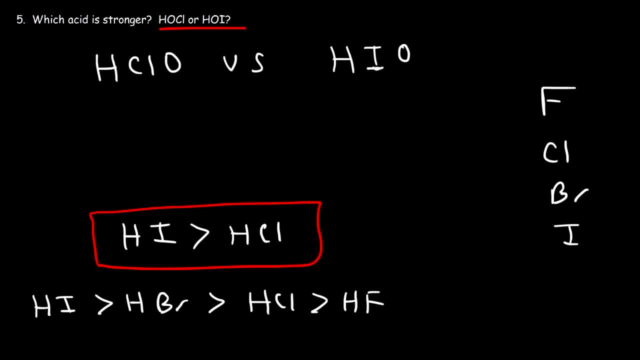 actually attached to the oxygen in these elements, So that trend does not apply. So it turns out for oxyacids: Acid strength increases Oxygen, Oxygen- Oxygen- Oxygen increases due to increase in electronegativity, So the trend is the opposite for this example. 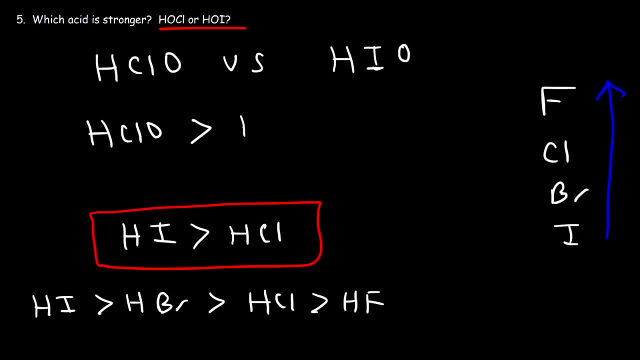 So what this means is that HDL O is the stronger acid than HIO because chlorine is more electronegative than iodine. So this is the answer. So make sure you understand this. For oxyacids, electronegativity is the main reason why HDL O is more acidic than HIO. 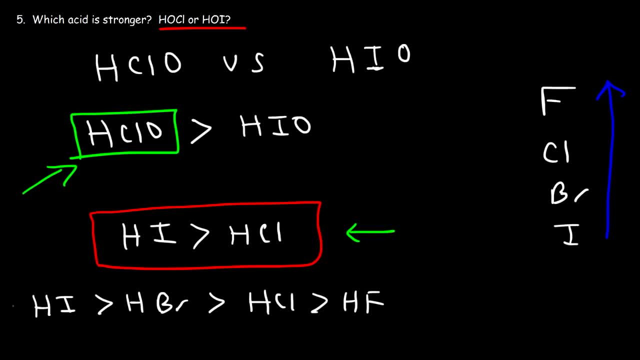 more acidic than HIO, But for binary acids it has to do with atomic size. The iodide ion is bigger than the chloride ion, and so the iodine ion is more stable. It can stabilize the negative charge better than the chloride ion can, And so it doesn't really need the 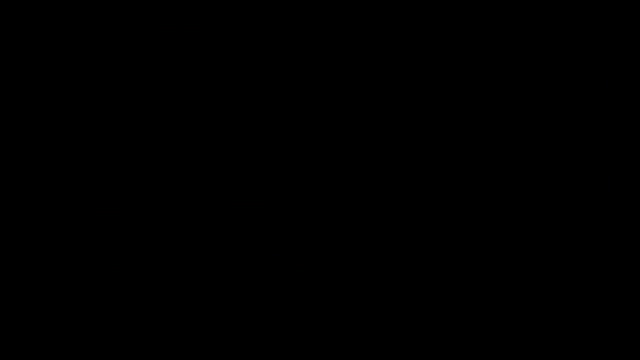 hydrogen to be attached to it, so it's more easier to ionize. So just to make sure you got that, which acid is stronger, HBr or HI? And what about HBrO versus HIO? Which acid is stronger? So for binary acids, the ones that don't have oxygen, acid strength increases. 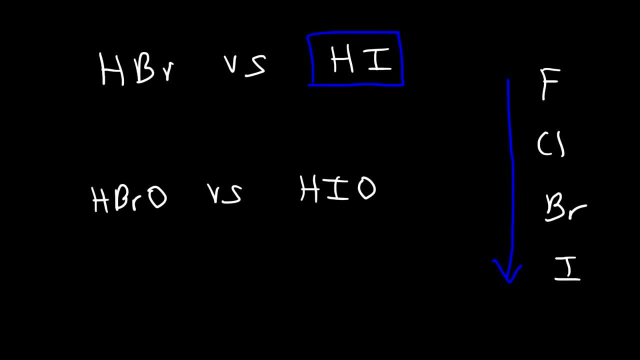 due to increase in size. So HI is a stronger acid than HBr. Now for oxy acids, the element that is stronger than HBr is HBr, So HBr is a stronger acid than HBr. Now for oxy acids, the one that's more electronegative is going to be the one that's associated with the. 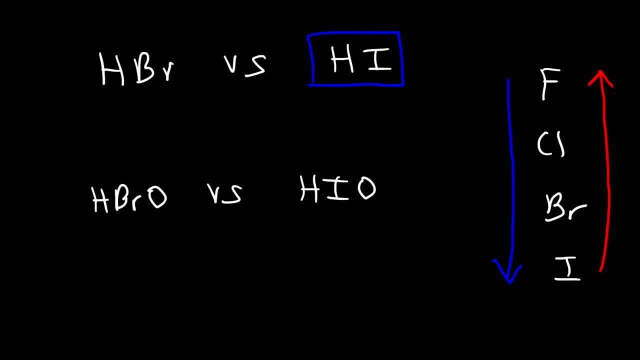 stronger acid. So bromine is more electronegative than iodine, So HBrO is a stronger acid than HIO. Number six: which of the following is considered to be a weak acid? Is it HTL, H2SO4,. 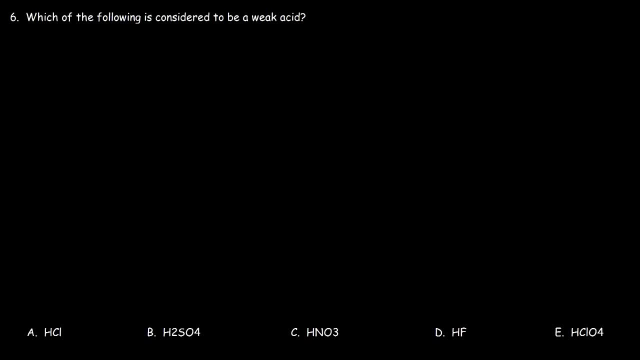 HNO3,, HF or HTL-O4?. Now it pays to know the six common strong acids, And these are HI, HBR, HTL, H2SO4,, HNO3, and HTL-O4.. So, if you're trying to identify, if 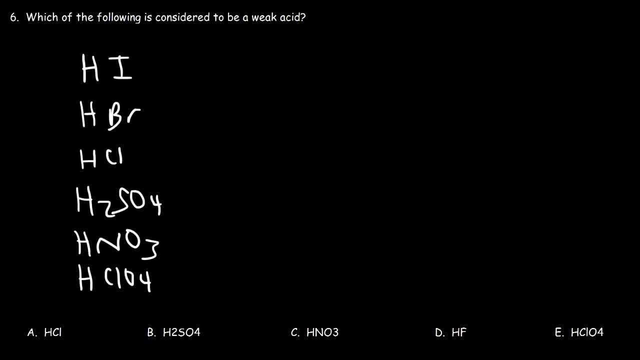 an acid is strong or weak. if it's not one of these six acids, it's safe to say that what you're dealing with is a weak acid. Now, it's not a hundred percent guarantee, but it's a good rule of thumb. So HTL is a strong acid. H2SO4 is a strong acid. HNO3 is a strong. 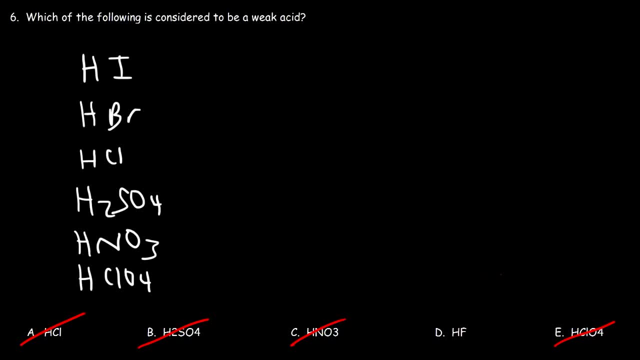 acid, And perchloric acid is also strong. So the weak acid is HF, hydrochloric acid, And that's the answer Number seven. which base is stronger, HS- or NO2-. Now we're given the Ka values for the conjugate acids. So for H2S the Ka value is about one. 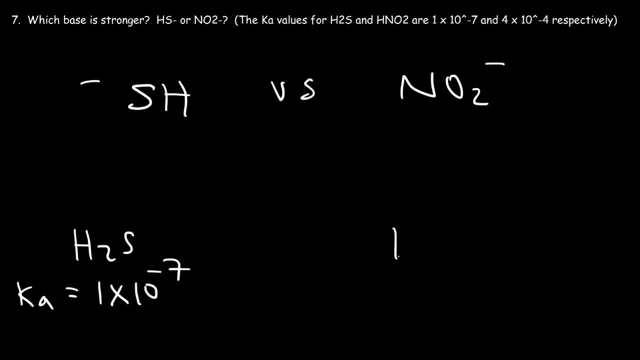 times 10 to the minus seven. And for HNO2, the Ka value is four times 10 to the minus four. So with this information, how can we determine which base is stronger? Now you need to know this rule of thumb: The stronger the acid, the weaker the conjugate base. So 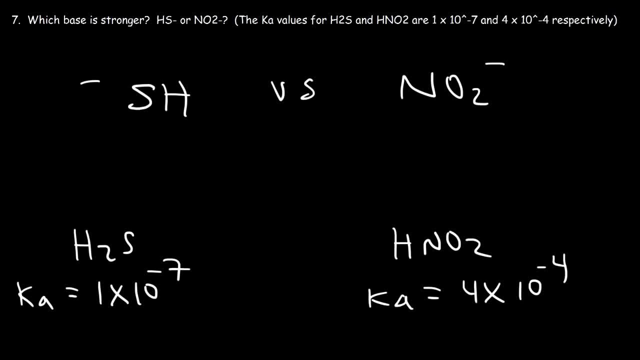 which acid is stronger, H2S or HNO2?. Negative four is greater than negative seven, based on a number line. So HNO2 is the stronger acid. So I'm going to write SA for stronger acid. That means that the conjugate base is going to be the weaker base, WB for weak acid. 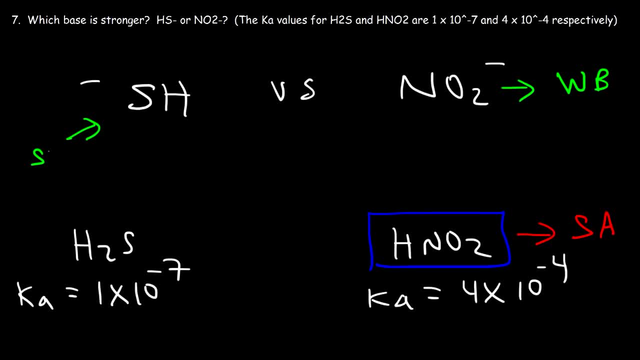 Which means this one has to be the stronger base because it's associated with the weaker acid. So the weaker the acid, the stronger the conjugate base, And the stronger the acid, the weaker the conjugate base. So we're looking for the base that's stronger. That's going.